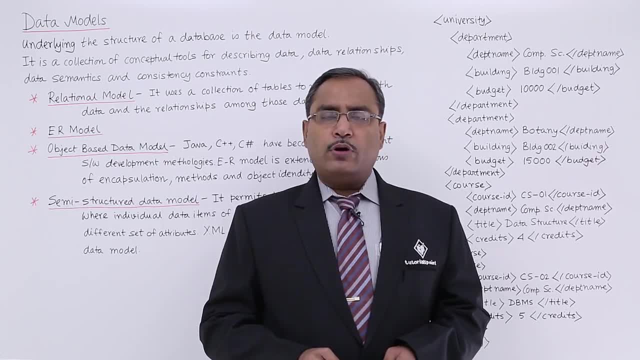 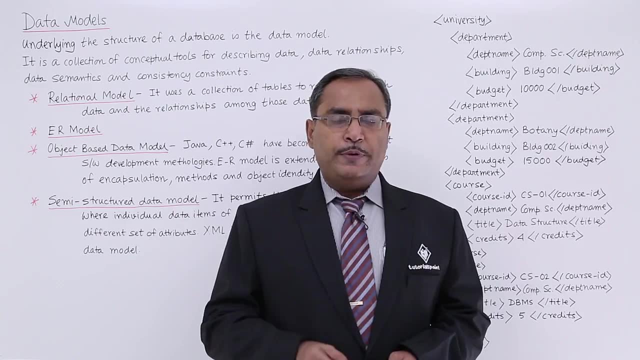 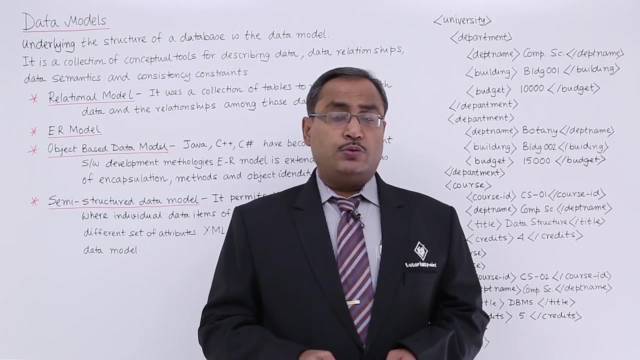 Let us discuss data model. This data model is nothing but a conceptual tool which will describe data, the meaning of data or the semantic of data, and the data relationships and representations. So it is very important and it is working as a underneath layer of. 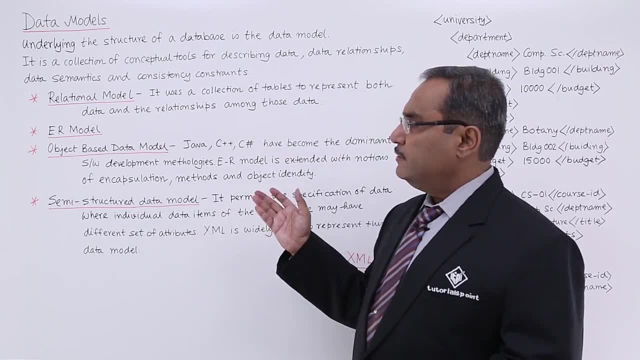 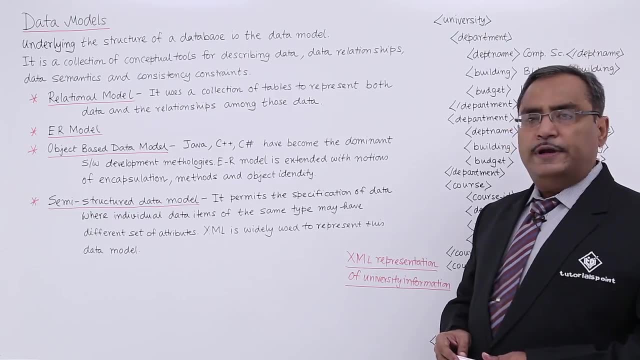 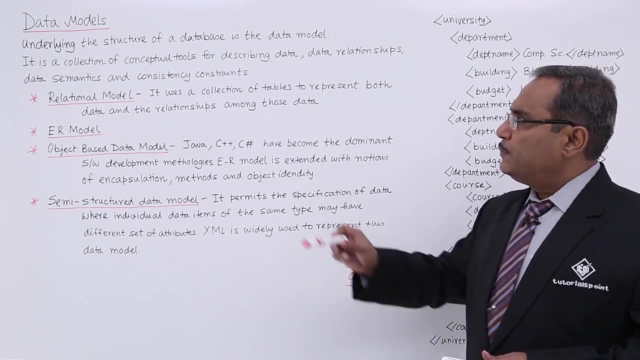 a particular database. So here is the classifications of different data models. So data model is underlying the structure of a database. So it is the underlying structure of a database. It is the data model and it is a collection of conceptual tool for describing. 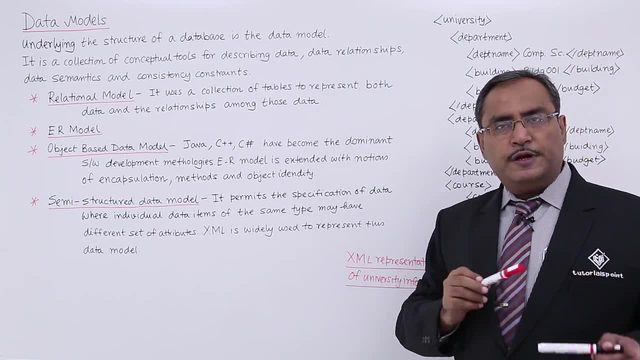 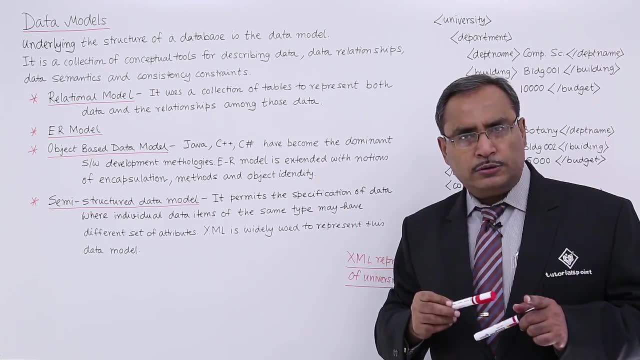 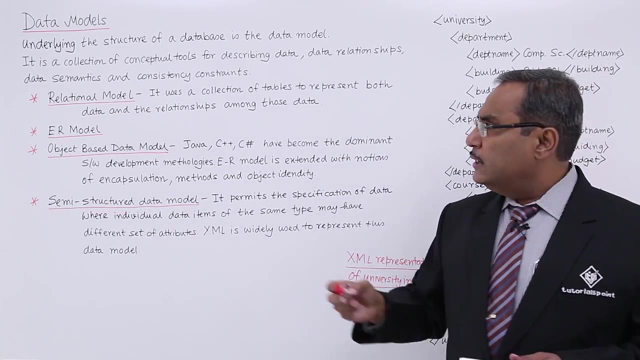 data, data relationships, how the different data are related, whether this particular data is related with data in another table or not. So there is a data, inter data relationships and data semantic. There is a meaning of the particular data and consistency constraints. So we are having 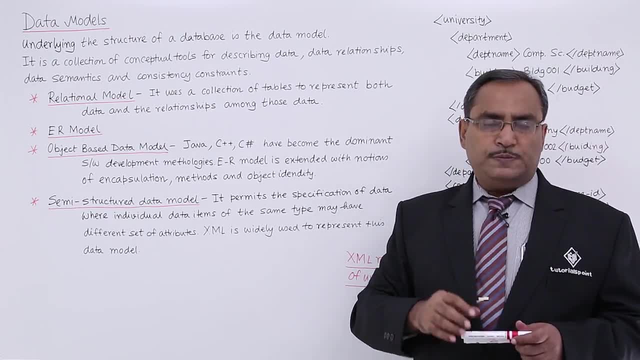 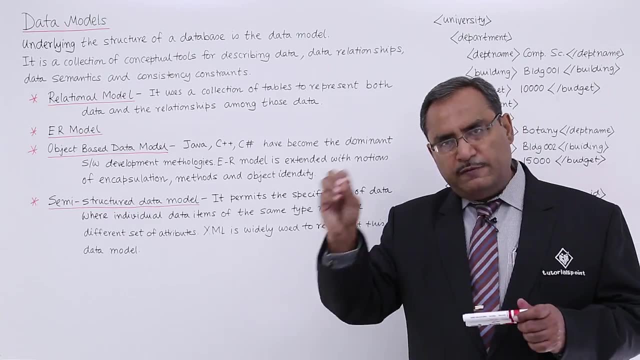 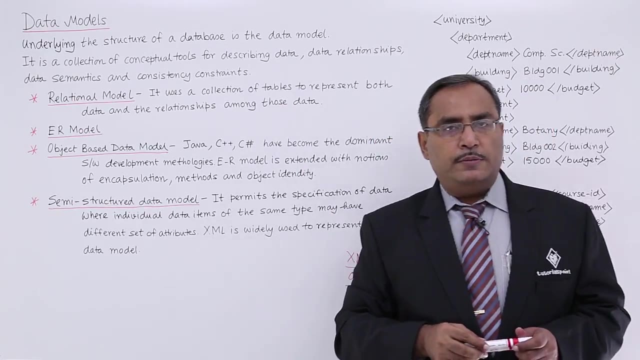 different consistency constraints will be there, So this particular data cannot be null. This particular data can be null, So this particular data must be faced from that very particular domain. So these are, the different consistency constraints are there, So all these things will be handled by this particular data model. Data model can be categorized. 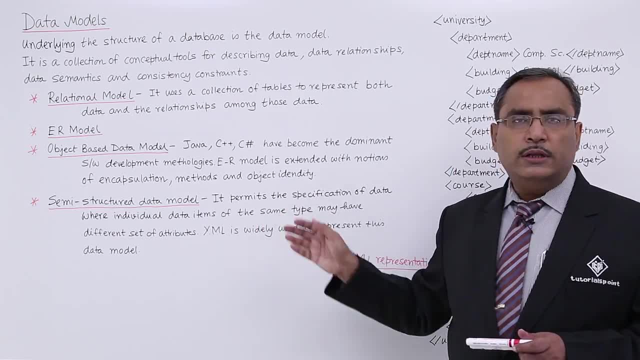 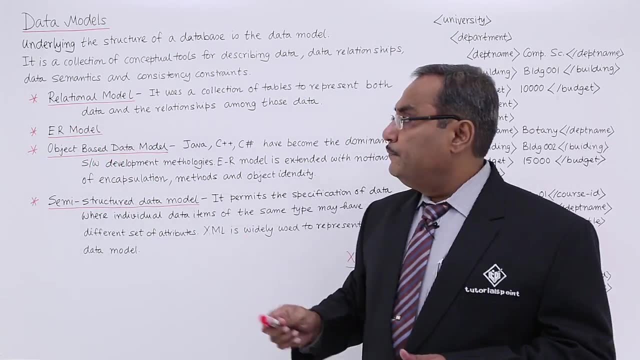 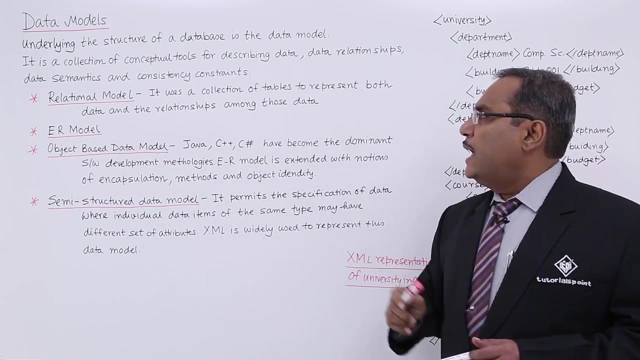 in multiple different ways. So here we have considered only the latest data models which we are dealing with nowadays. First one is a relational model. It uses a collection of tables to represent both data and the relationships among the data. So in case of relational model we are having 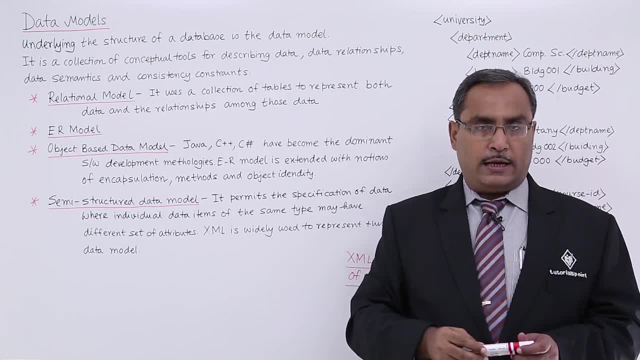 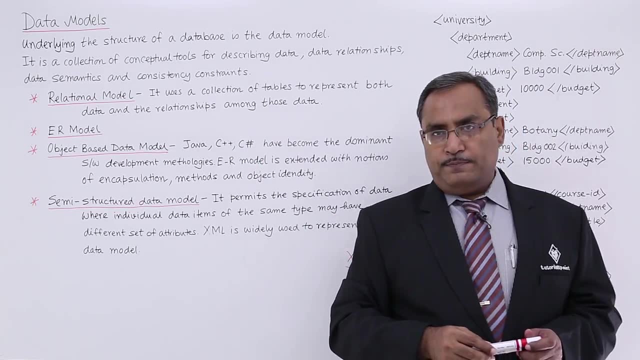 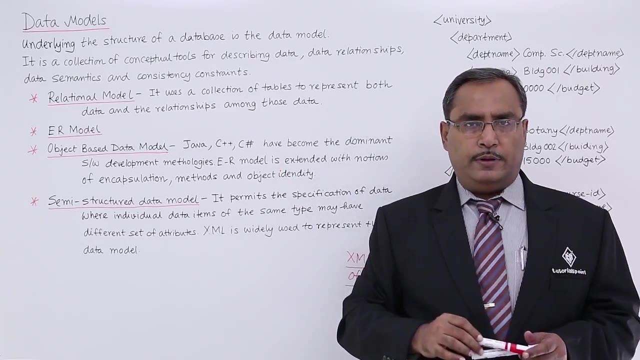 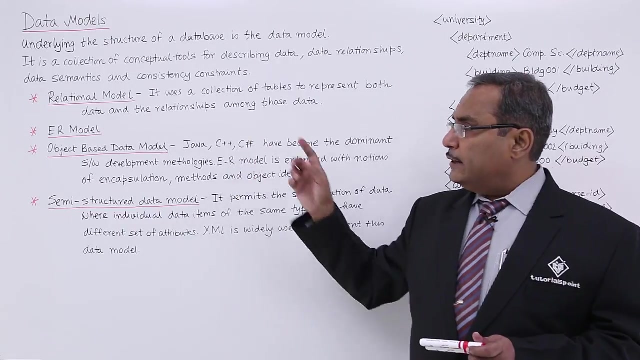 collection of different tables. Those tables will be holding data and this particular tables will represent data and also the relationship between the data. So in case of relational model, we are having, say, one table where one attribute is common with attribute in another table. So through those attributes these two tables are related and we know that. 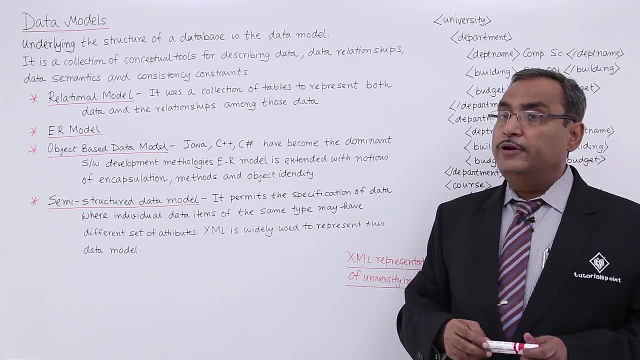 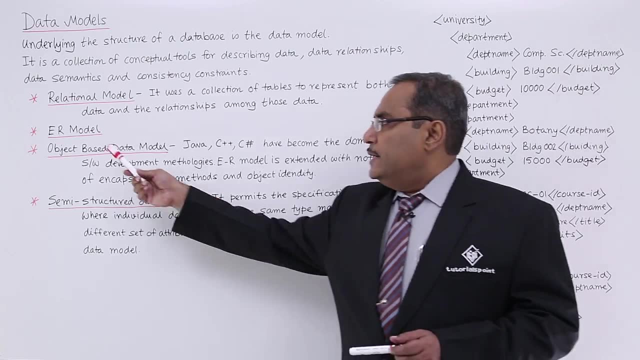 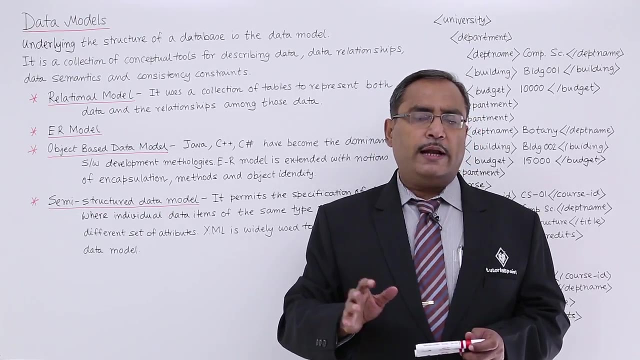 in case of relational model, tables are also known as relations. The relations are the other names of the tables, So tables can also be called as relations ER model- full form is entity relationship model. We will be having a separate video on this ER model and their detailing and different 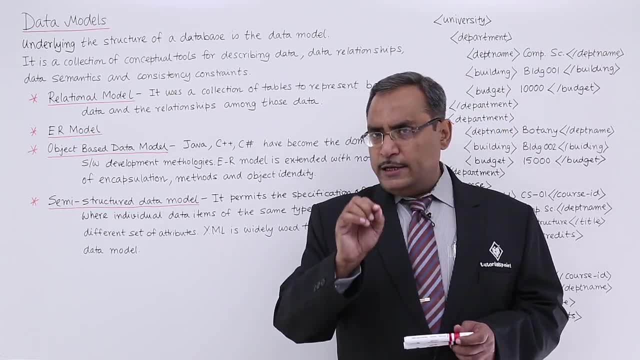 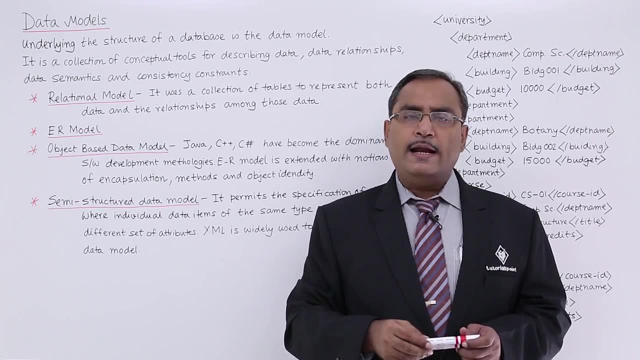 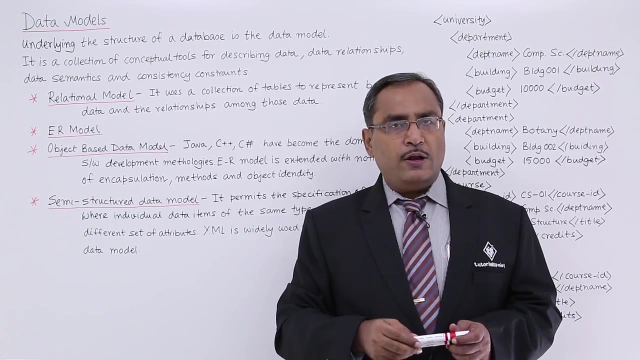 aspects of this ER model. So it is entity relationship model. Entity means which is something which is having a permanent existence in an enterprise With an entity. some set of attributes are connected. Depending upon the values of some attributes, an entity can. 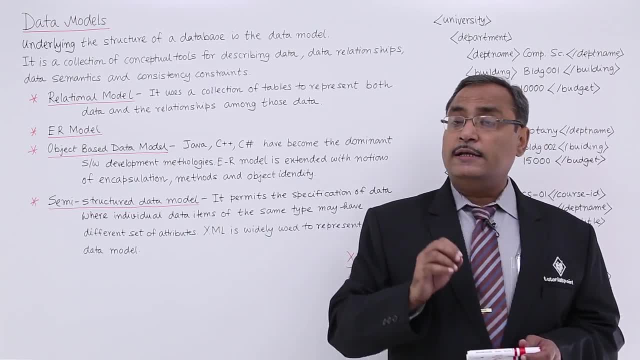 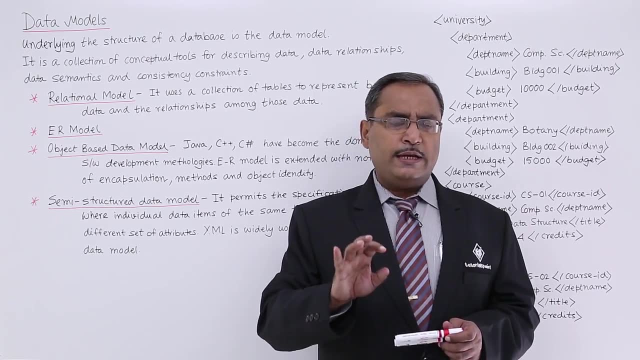 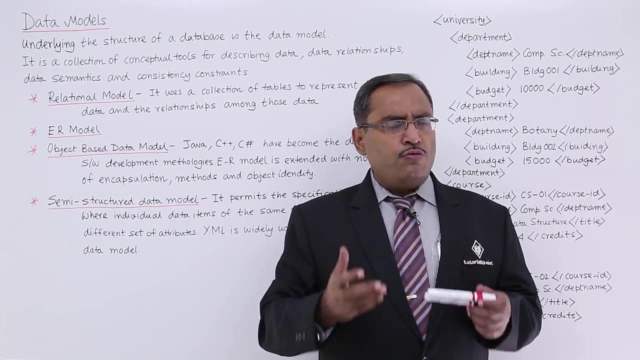 be identified uniquely. So that is the definition of entity relationship model. An entity will have a permanent existence in an enterprise. Let us suppose in a college there is a particular course, So course is an entity. It might be true that for a certain 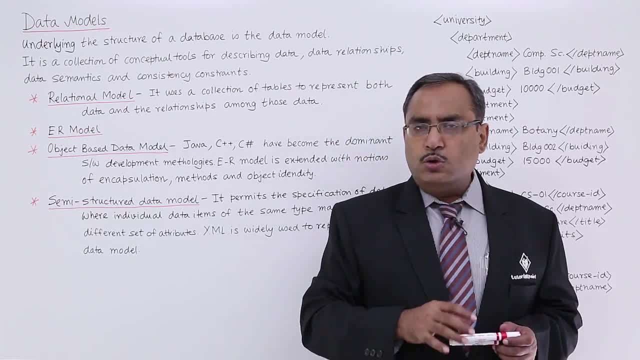 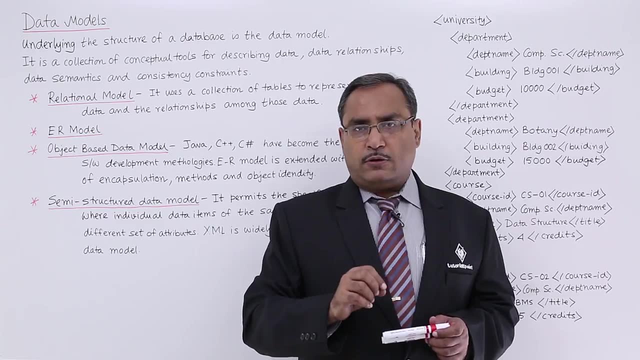 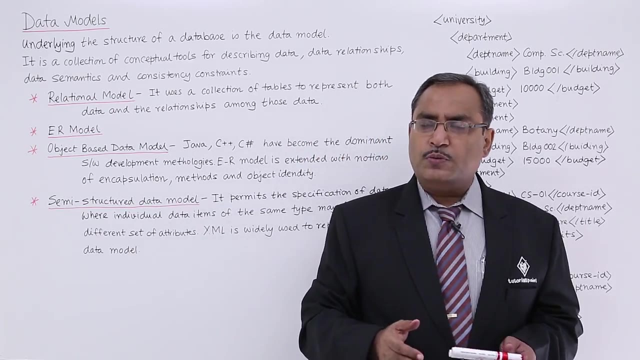 course there is no admission. for the last 6 months, No student has taken any admission to that very particular course. In spite of that fact also, the course and its respective details will be kept in the course 0 course table. So that is why course is an entity, permanent existence, And course will have the 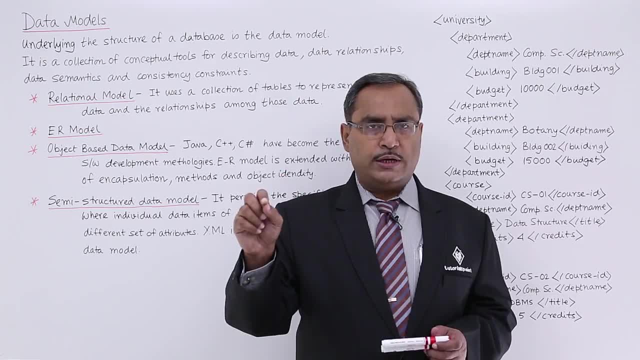 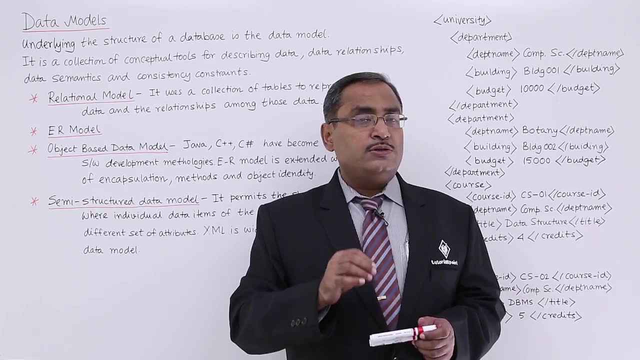 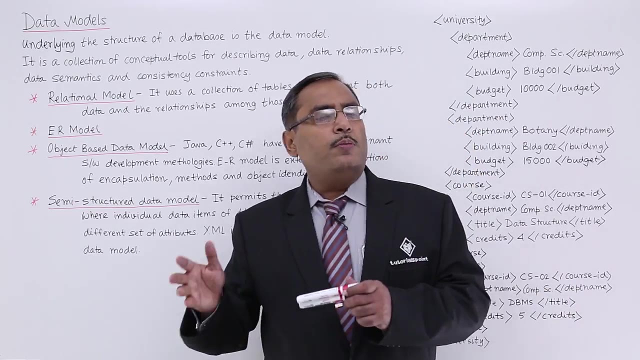 course, ID course, name course, phase, course, duration and other details. So these are the set of attributes which will depict that particular course. So this is known as an entity, And relationships will denote the relationships between two or more than two entities. So 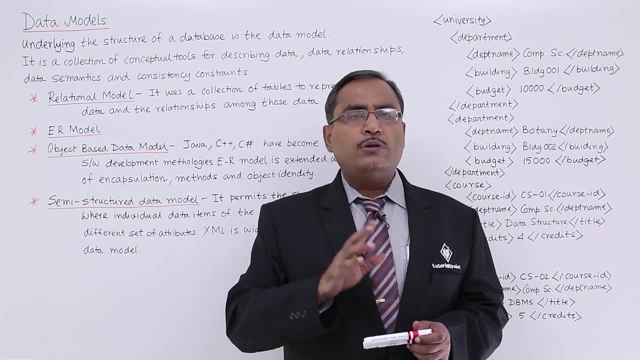 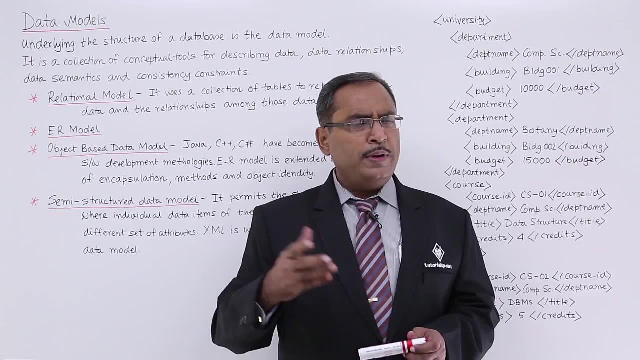 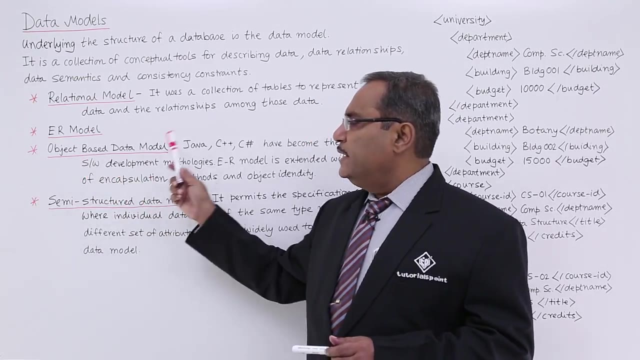 that is a relationship, How the entities are related, how the entities are having the relations in between. that will be depicted in the relationships. So we will be having our detailed discussion in the respective videos. on this very particular data model, We are having object-based data model. We know that nowadays Java, C++, C, hash have 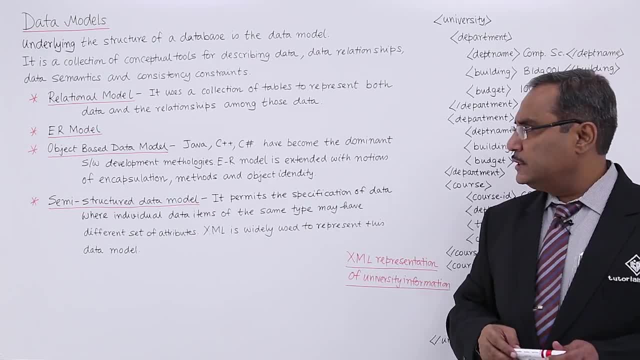 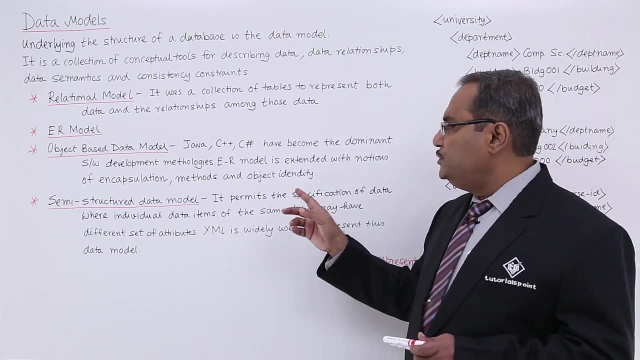 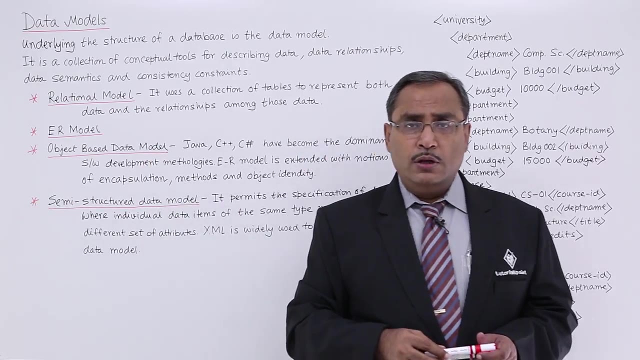 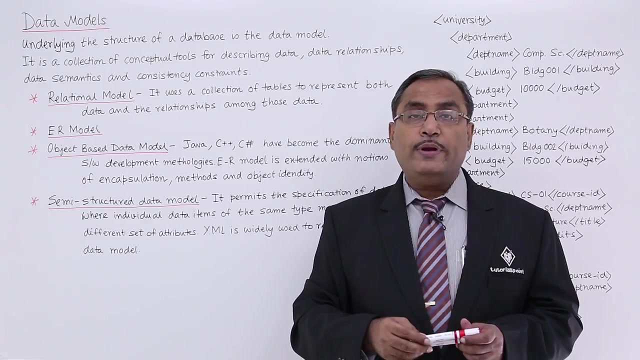 become the dominant software development methodologies. Year model is extended with notion of encapsulation methods and object identity. So now we know that in case of this particular object-based data model, here we will be having methods which will be denoting that what are the permissions, permitted operations that we can carry out on a set of data and 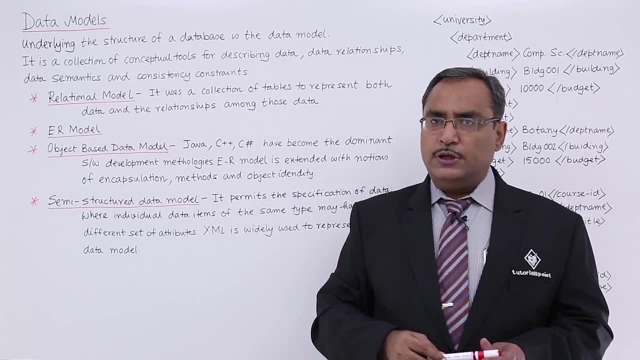 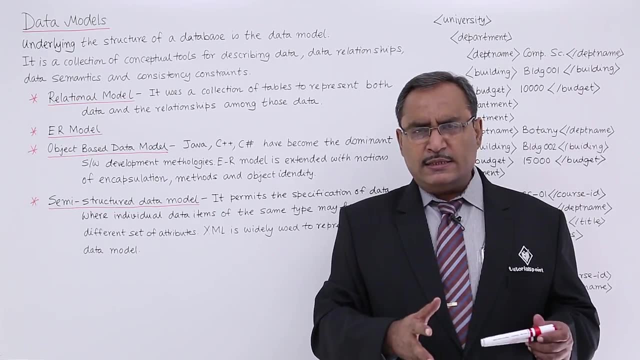 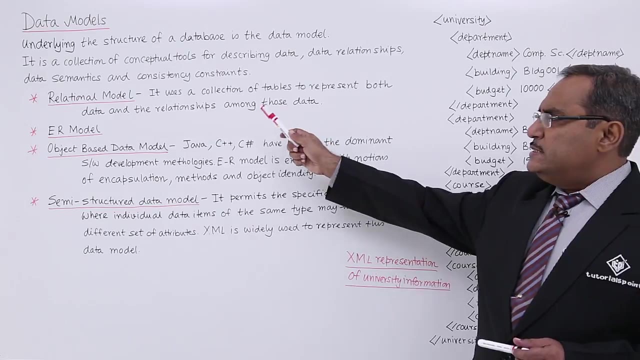 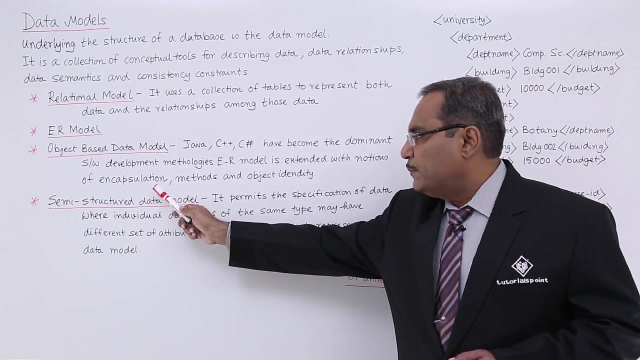 this particular data are nothing but the variables. So these particular operations, that is, the methods, data known as the messages, so that will form this particular object based data model. this year model has got its object based data model version as your model is extended with notions of encapsulation, methods and object. 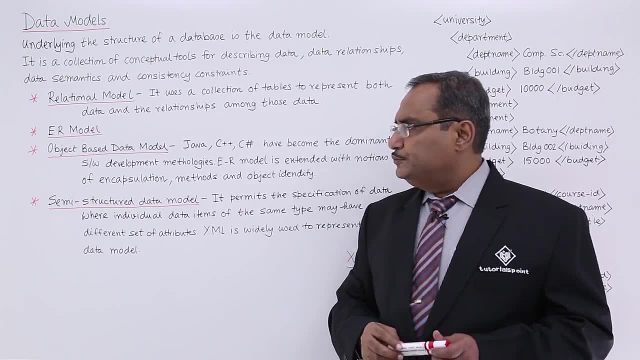 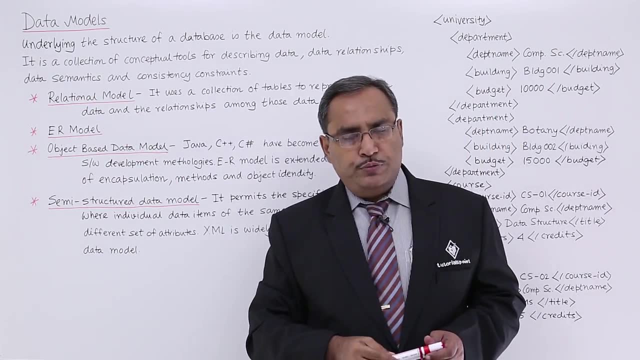 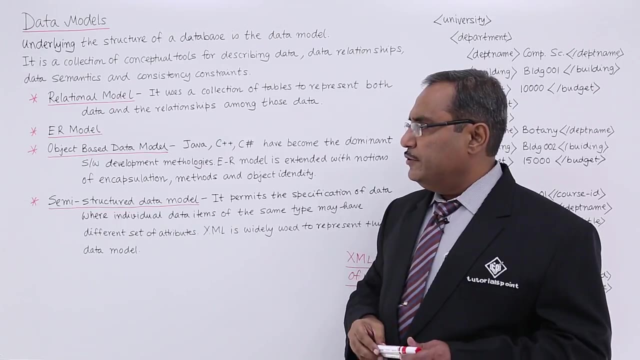 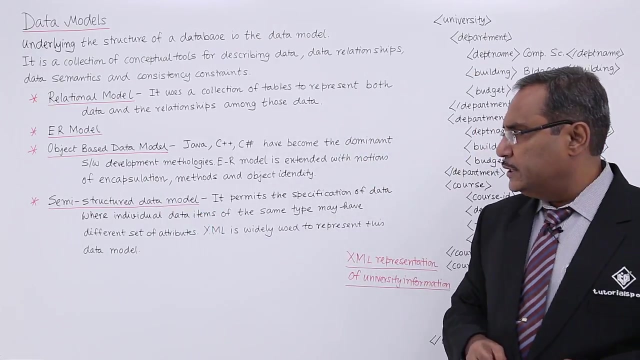 identity. so of also, we're having object relational data model, so this data model is also having the object oriented flavor, and thus the new data model, the new version of this relational model is object relational data model have been invented. so now the last data model which we are going to share here is the semi structure data model. 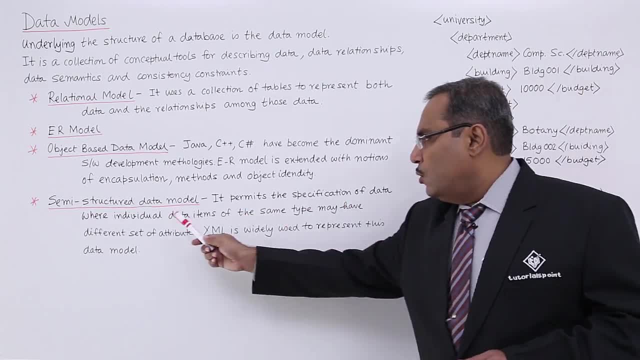 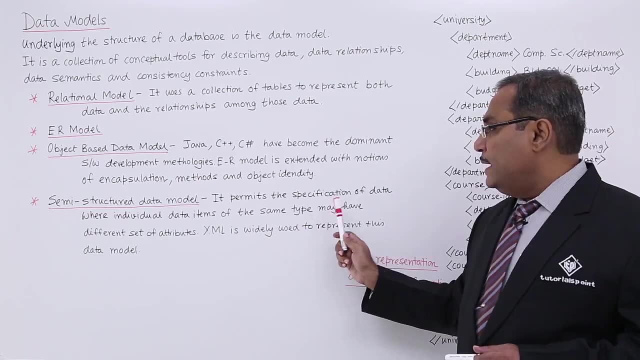 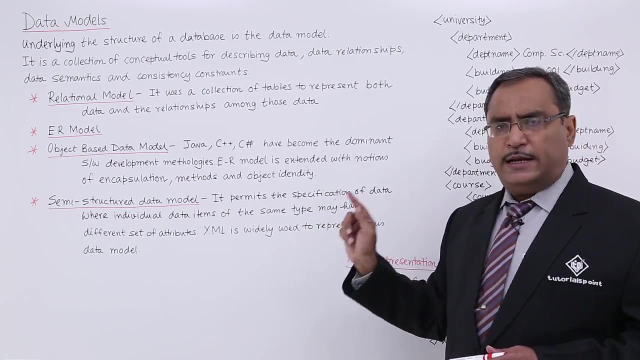 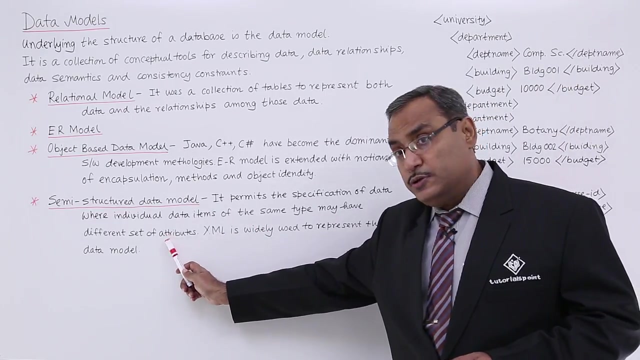 it permits the specification of data where individual data items of the same type. so individual data items of the same type may have different set of attributes. so a particular specification of a data will have different set of attributes. same type may have different set of attributes. so that is very important. 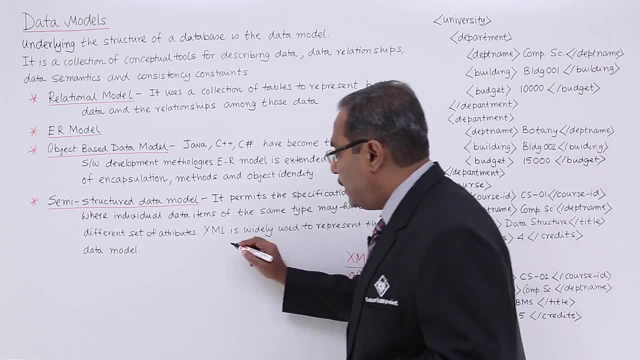 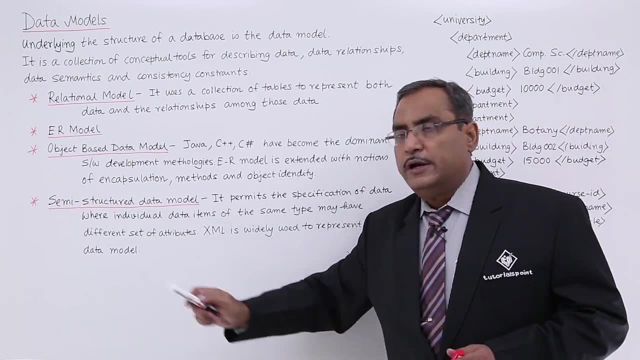 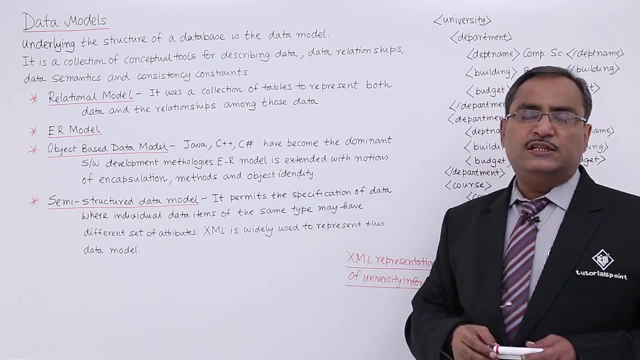 and xml. xml means extensible markup language, so xml is widely used for the use to represent this particular data model. so xml- that is the extensible markup language, is, is, is, is- is widely used to represent this particular data model. so to have the better clarity on this particular topic, let us consider this. 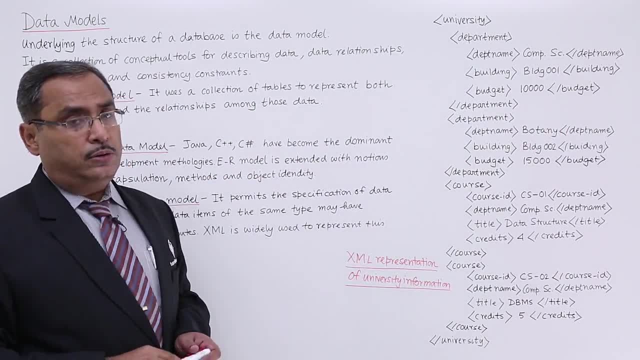 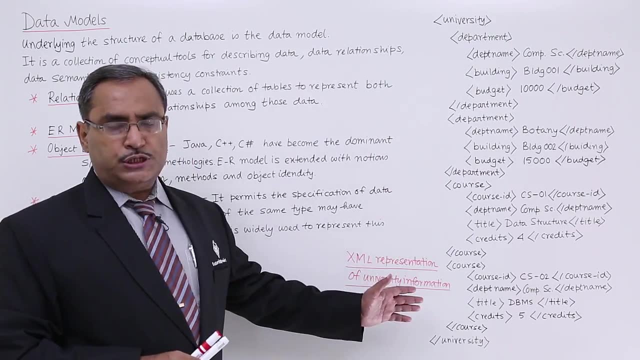 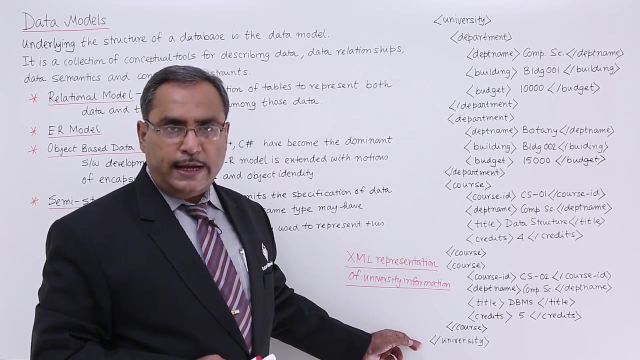 particular course segment of this particular xml and it is a xml representation of university information. obviously it is a partial information we have demonstrated so this is the university and this is the slash university. so this is the closing tag and that is the opening tag. now, under this, we are having this: